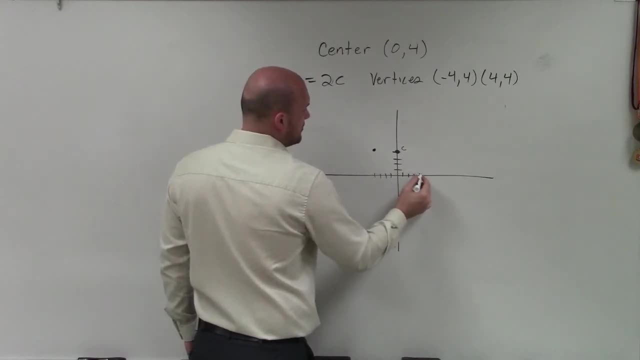 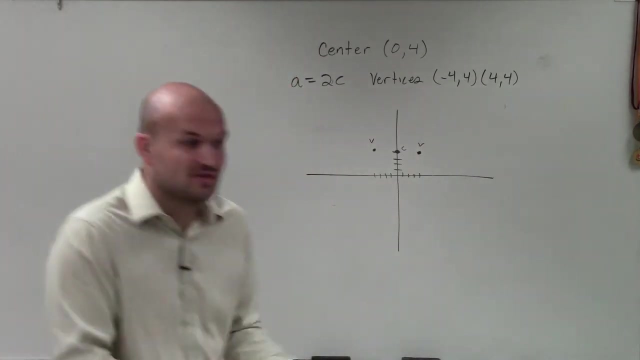 4. And positive: 4,, 1,, 2,, 3,, 4, up, 1,, 2,, 3,, 4.. OK, Now, those are the two vertices. Now remember the vertices. the foci and the vertex all lie on the major axis. Very good, 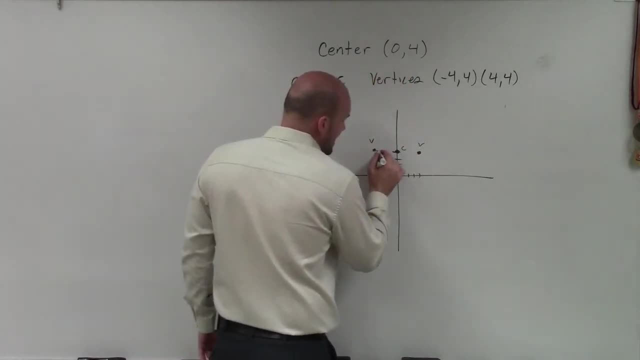 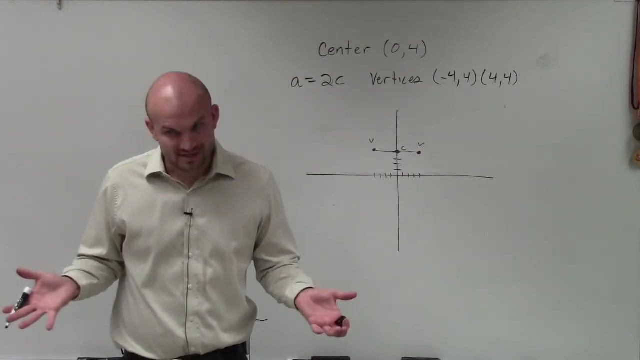 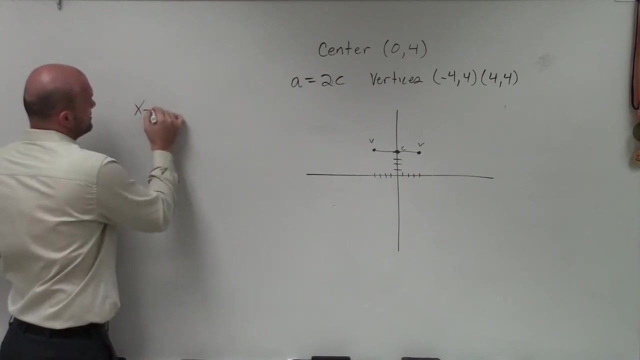 So if they all lay on the major axis, that means we know the foci are going to lie on this as well. But now I'm going to have a major axis that is horizontal or vertical, Horizontal. So therefore, to determine which equation I'm going to use, I have to use this. 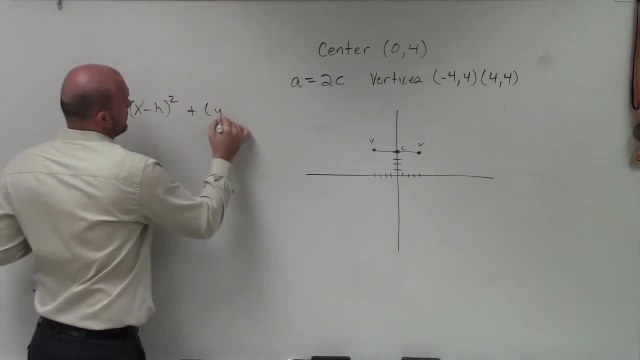 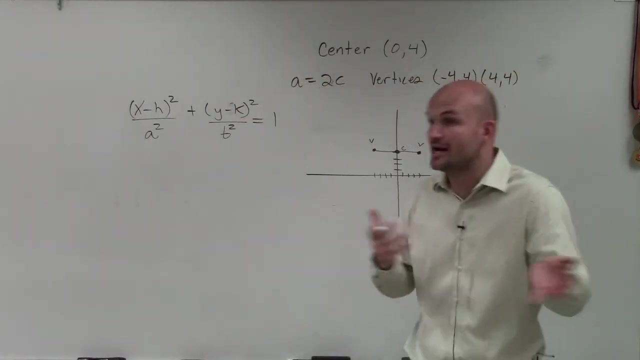 equation Where a squared is now going to be under the x and b squared is under the y, and that's equal to 1.. Do you guys understand how it has to be that equation, not the other? Because you have to choose. The only way you're going to understand how to choose is to graph the. 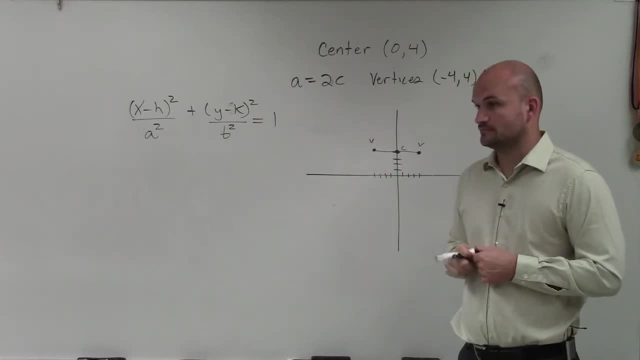 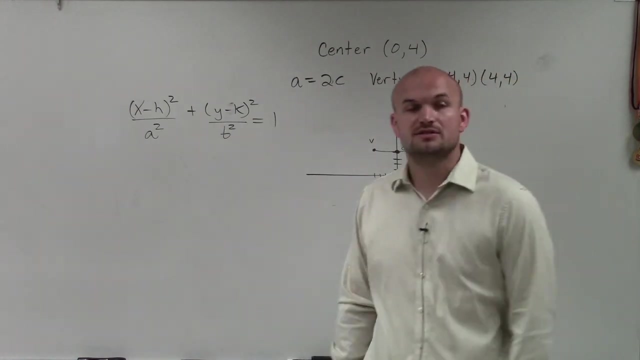 information you have. Yes, So like, since h and k is the vertex, what is the h and k? There's no vertex. h and k is your center. There is no vertex for an ellipse. We talk about our center. So, yes, h and k are going to represent the center for your. 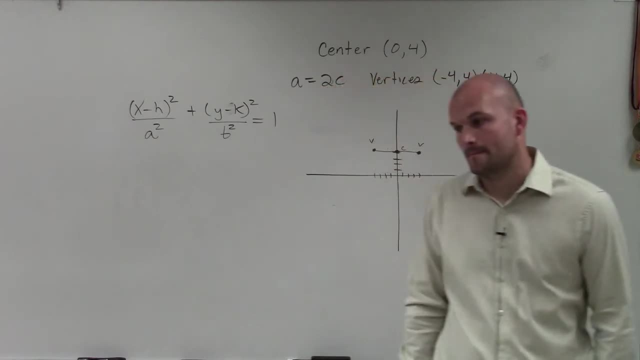 ellipses. I believe in the problem. The center says 0,, 4, 2, negative 1 for question 42. So you did what I did. anyway, I did the same thing, but I did 45, so don't worry about. 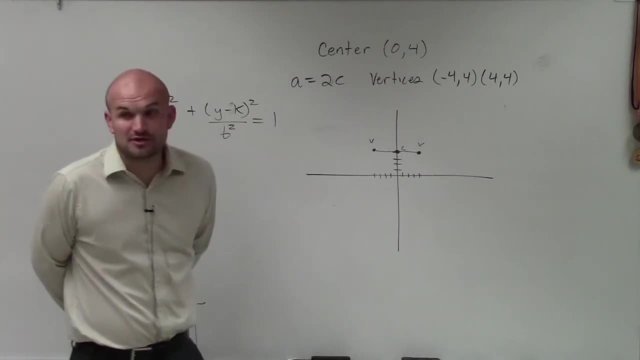 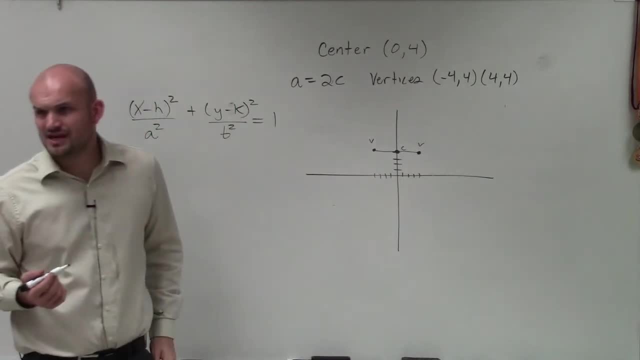